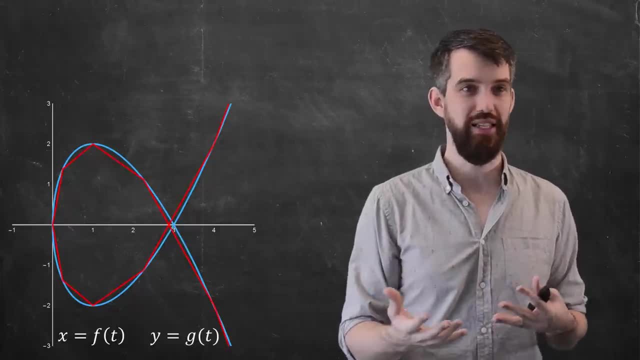 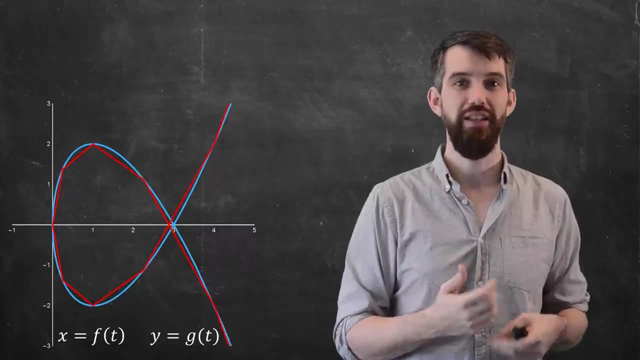 a bunch of straight lines, And the basic reason for this is that straight lines are things I know how to compute the length of and I can sum up all the straight lines and maybe take some sort of limit. So the sort of guiding philosophy for our formula here is that the arc length 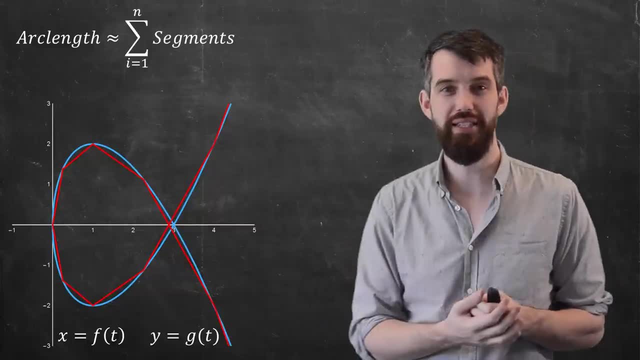 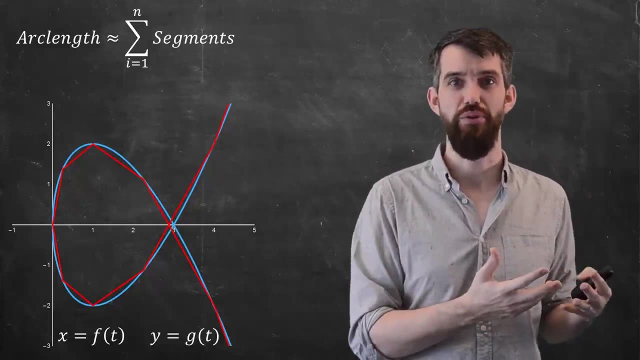 is going to be the sum of all of these little line segments and I can figure out the length of any individual line segment. Then I'm going to take the limit, as n goes to infinity. so the number of segments gets very large, but the length of any individual segment gets smaller. 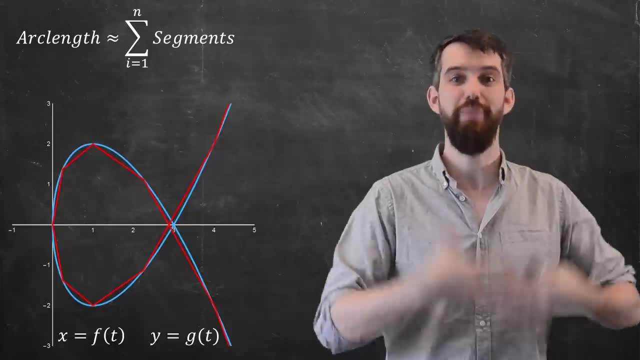 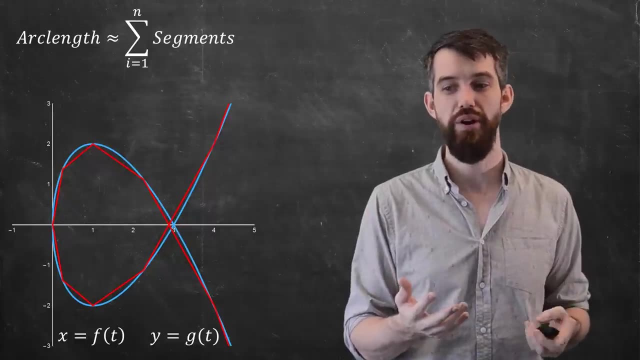 and smaller and smaller, And then, if I do that, I replace my summation with an integral, and well, that's how we did arc length in the past, So let's do that again here. So first thing I want to do is I really want to zoom in on one particular region here, So let's just talk about one little. 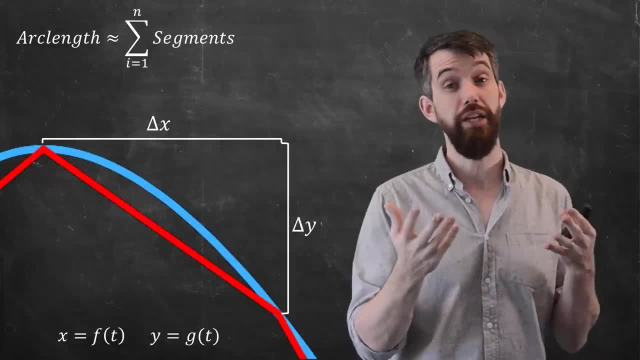 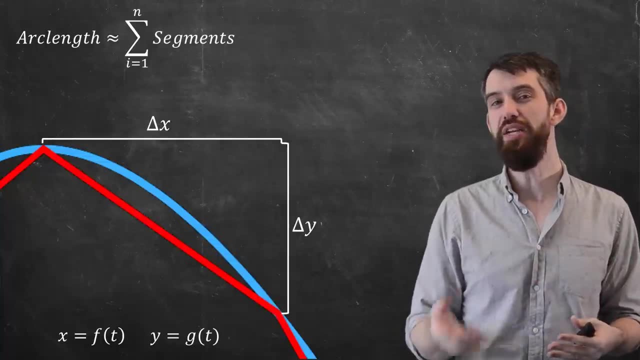 region of arc length. I've got to change an x and I've got to change an y. Now, in the past, when we talked about arc length, we talked about arc length as a function of t and y. What we did was we took the x and we divided that up into n different little regions, the 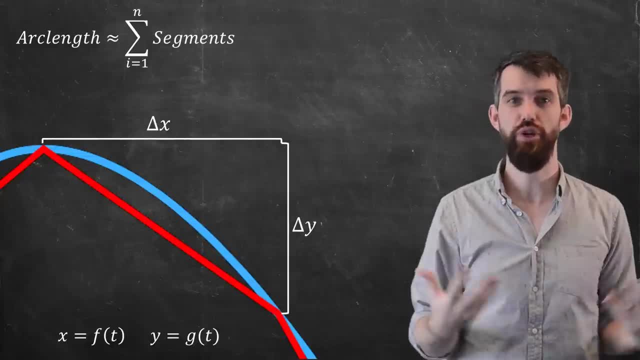 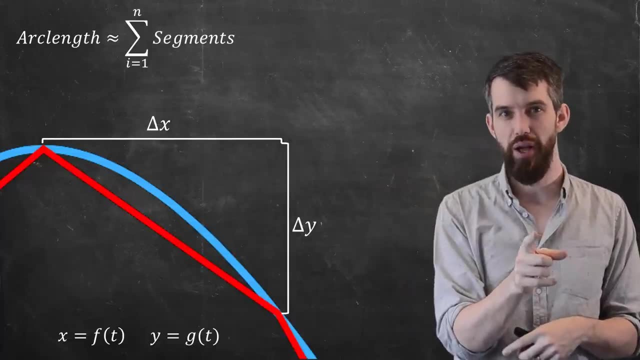 regions that each have a width- delta x. And then what we focused on is: well, what is delta y? and it was going to be the derivative of the function times, delta x, But in this video, well, both the x and the y depend on t. so the thing we're going to break up into 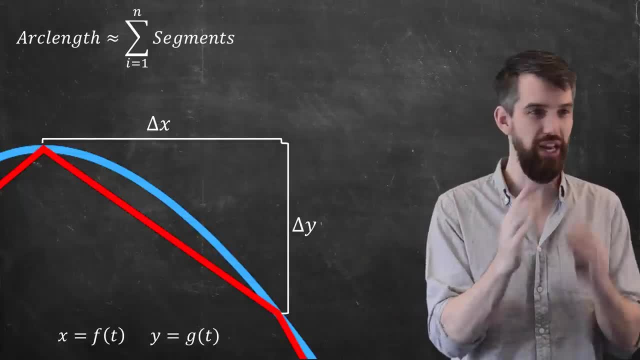 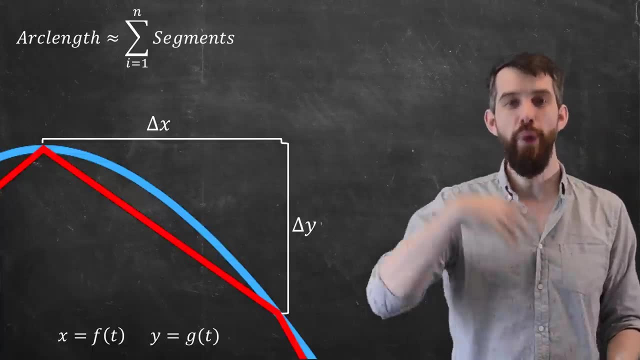 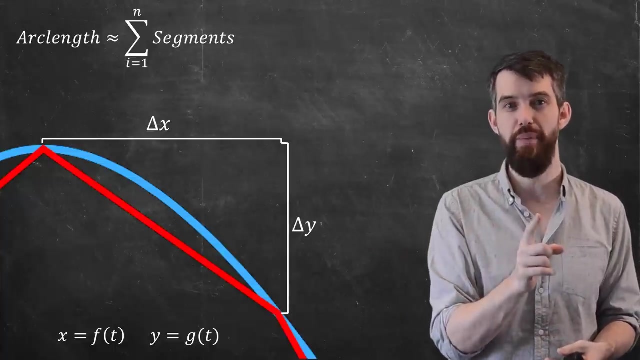 a bunch of little regions is not the x's, it is the t values, that you have some interval of t's. you break that up into n different regions. So what we're going to do is we're going to take delta x and I'm going to write this: 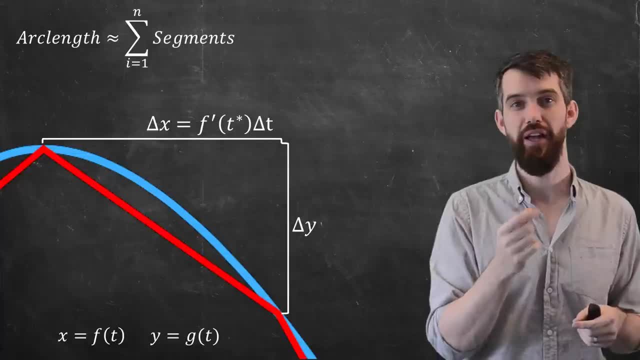 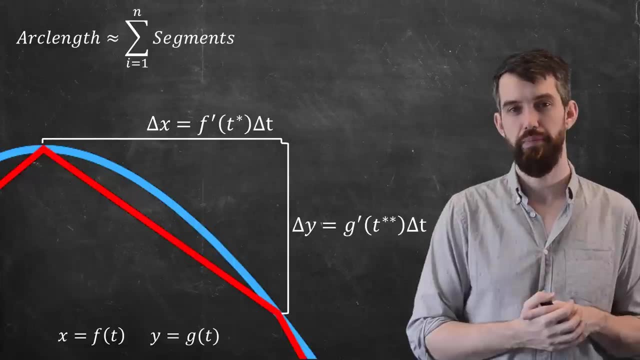 as the derivative f prime- remember x- is equal to f times delta t, And then my delta y is going to be g prime times delta t. Now why do I have a t star and a t double star in there? Why do I have a t star and a t double star in there? The reason is the same reason we. 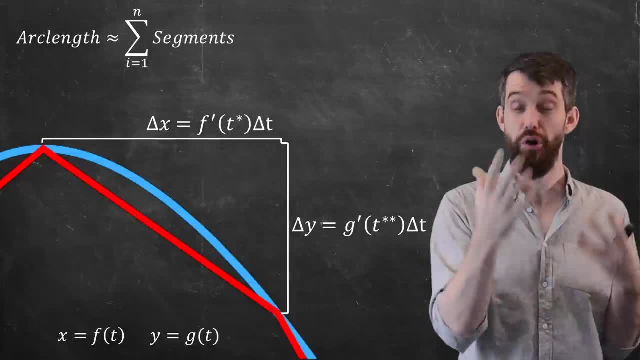 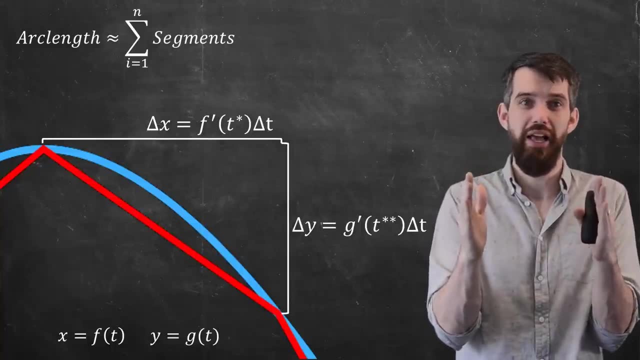 had a star back when we did arc length the very first time earlier on in the semester. And basically what we're doing is we're doing a mean value theorem here And what we're saying is that in this little region there is some spot in the middle of that region. 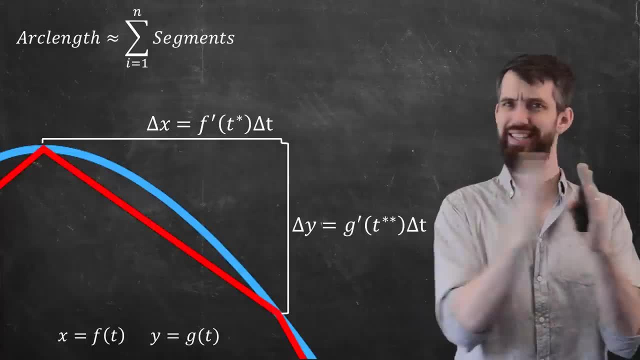 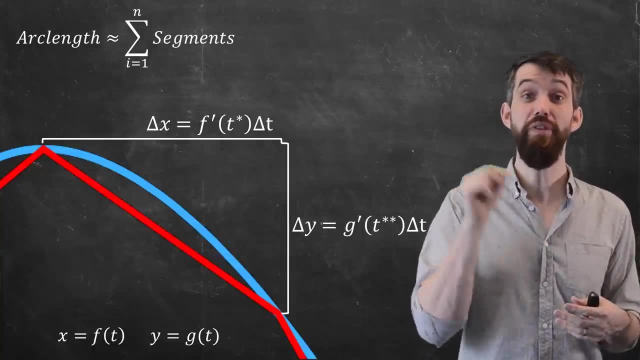 I don't know exactly where. so that's why I put the star there. Star says it's somewhere in there, but I don't know where. And then what the mean value theorem says is that at that particular point the slope of the tangent line was equal to the slope of the secant. 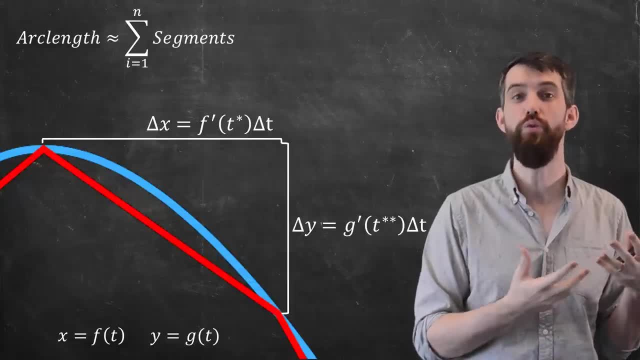 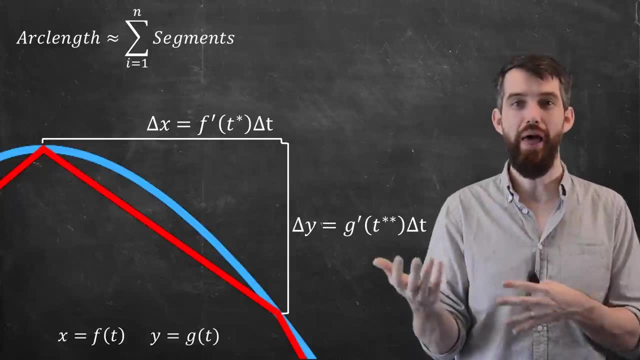 line, Or in other words the discrete slopes like delta y over delta t, was just equal. It was equal to the derivative of the actual slope of the tangent line at some point in the middle. Now, none of this is going to matter all that much because we're going to take a limit at 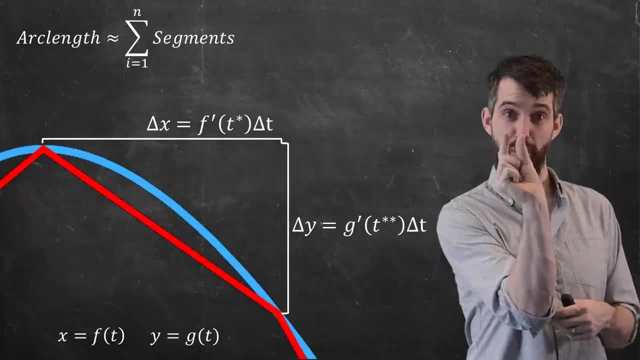 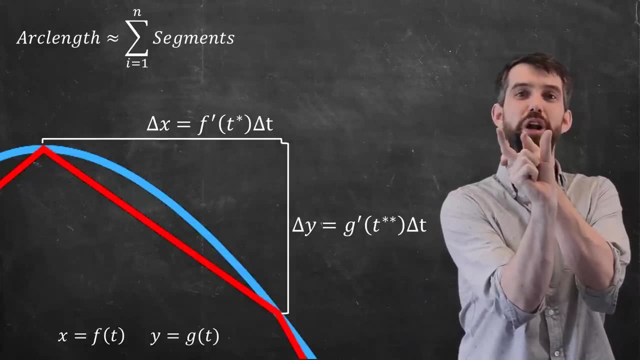 the end of the day, And what we're going to have is our delta t is going to go smaller and smaller and smaller, and the limits become infinitesimal. So the fact that we don't know exactly where this equality occurs is not going to be relevant when we take our t and 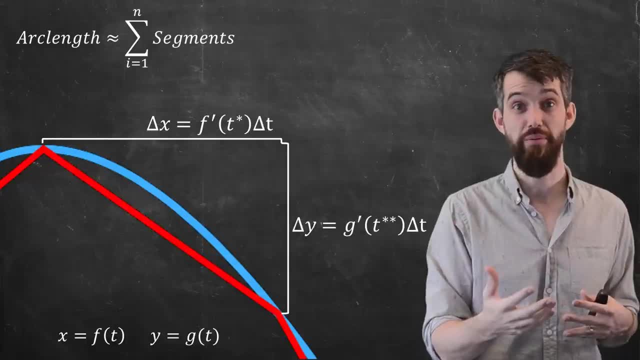 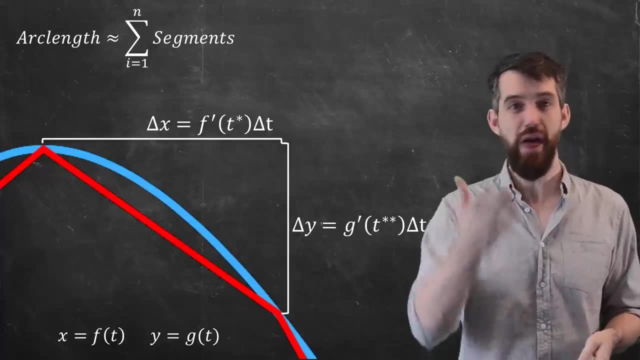 send it down to zero. Now, the thing we actually care about is the red line. here. We want to know what this straight line we're trying to approximate that. Well, this is nothing but by Pythagoras, the square root of delta x squared plus the 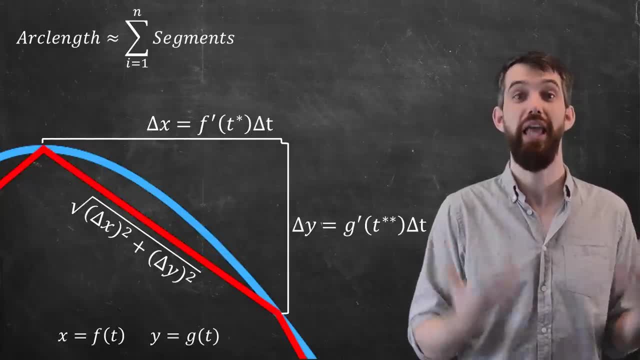 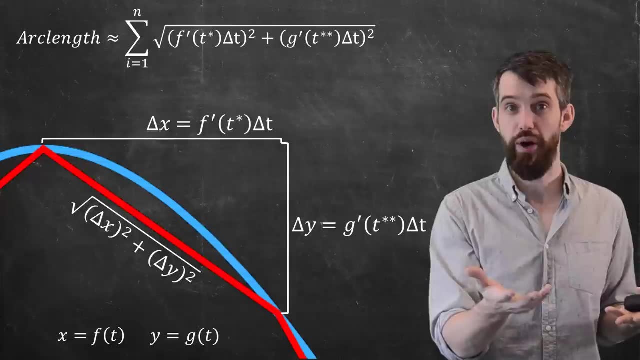 delta y squared. Okay, so that's what I'm going to put in for the length of my little line segment. So what do I have? This is the summation of the square root of, first of all, the delta x squared. 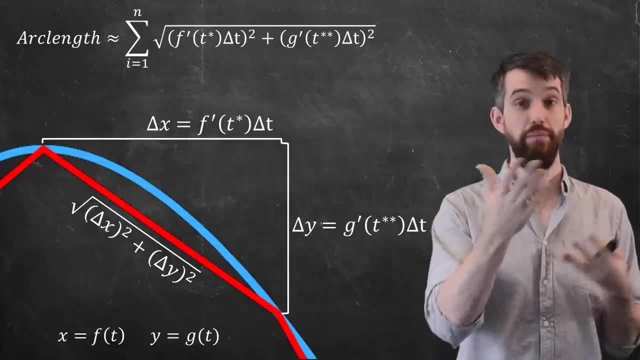 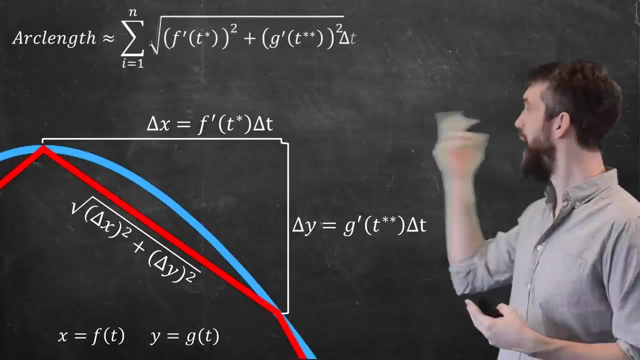 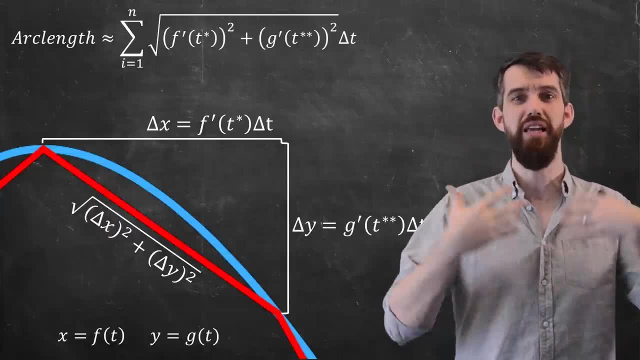 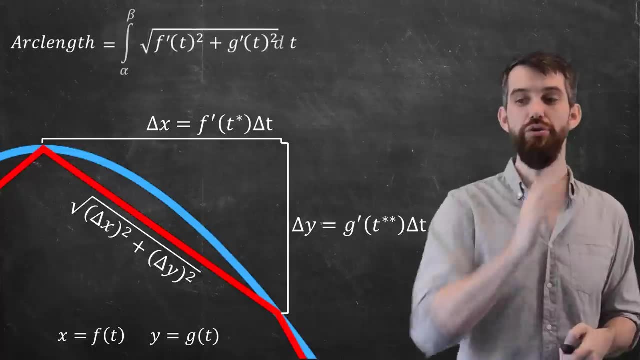 I'm going to do that, I'm going to do that, I'm going to do that. Then my final trick is the most important. It's the replacing the summations and the finite deltas with a limit, as n goes to infinity, and that gives me an integral sign all the way out the front. 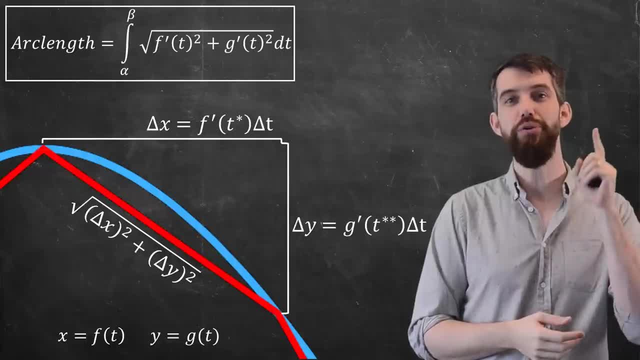 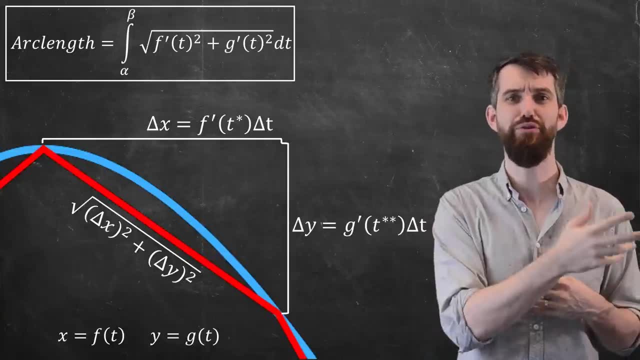 an integral, from alpha up to beta, of the square root of f prime squared, plus g prime squared. all of that in integral dt. Alright, so now that we've sort of sped through re-deriving arc length in this new context, let's actually see an example. So let's go back to the familiar one. we've seen a couple. 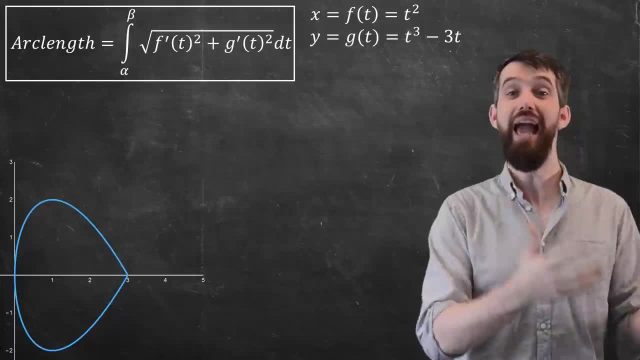 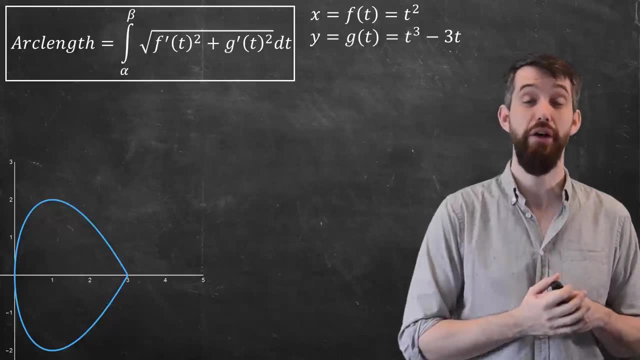 times now, This particular curve where what do we have is x is t squared and y is t cubed, minus 3t, And I'm in particular going to focus on just the loop. That's what I want- to figure out, the arc length of that loop. Now I'm going to need both derivatives, so f prime is 2t. 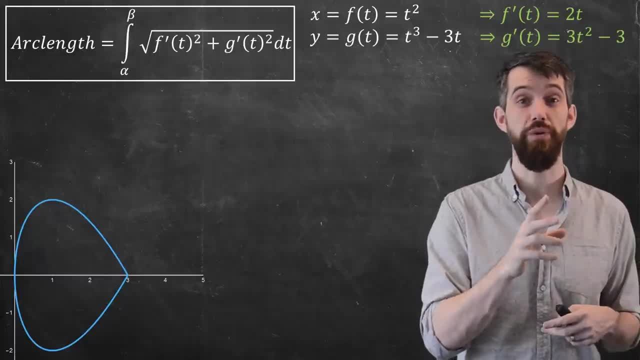 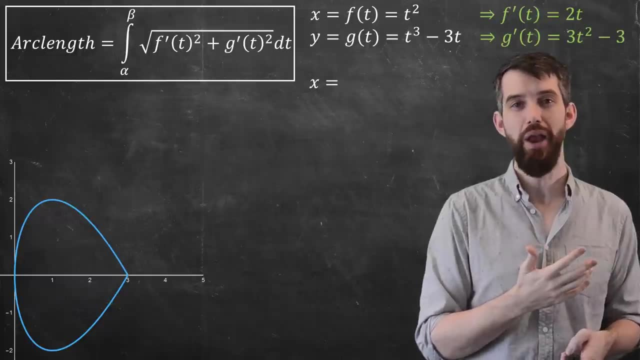 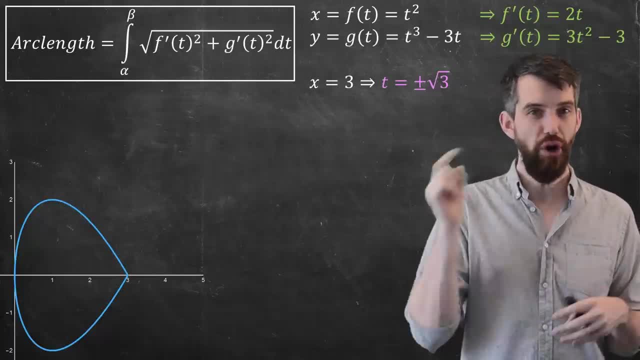 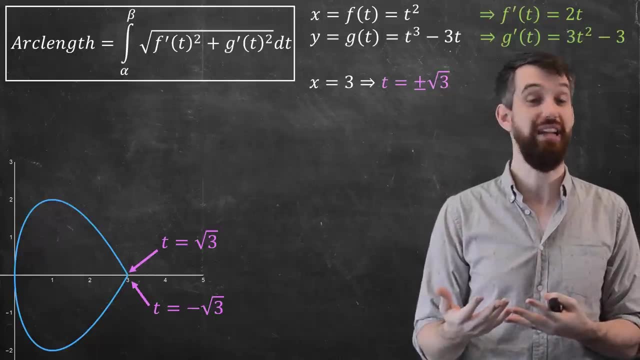 So what I'm doing is I'm starting: 2x is equal to 3.. I'm going all the way around my loop and getting back to x is equal to 3, but it's at two different t-values. I could start at: 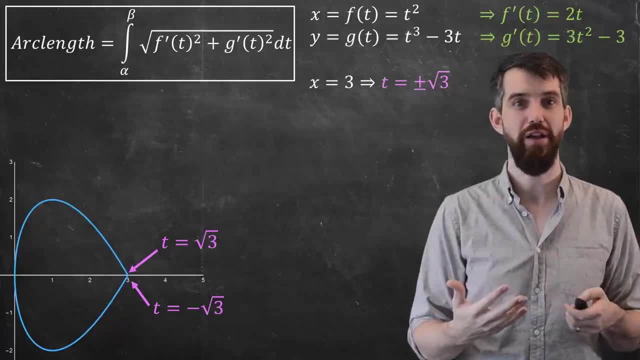 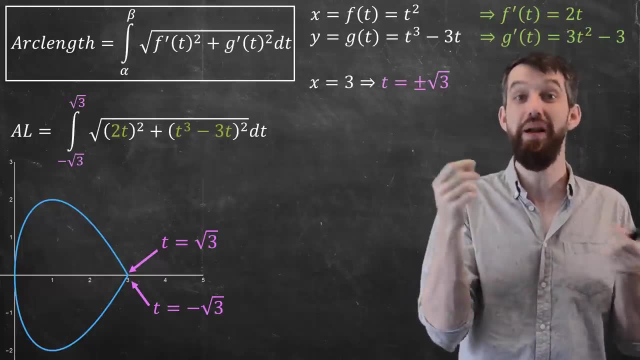 say minus root 3 and go up to plus root 3.. So if I'd plug all of that into my formula, what do I have? The integral from the minus root 3 up to the plus root 3, the two sort of endpoints of my interval of t, And then I'd plug in my 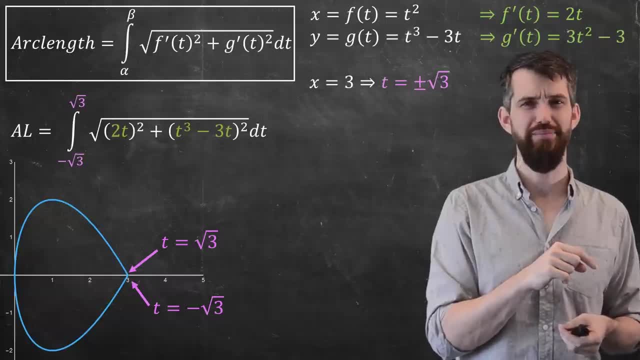 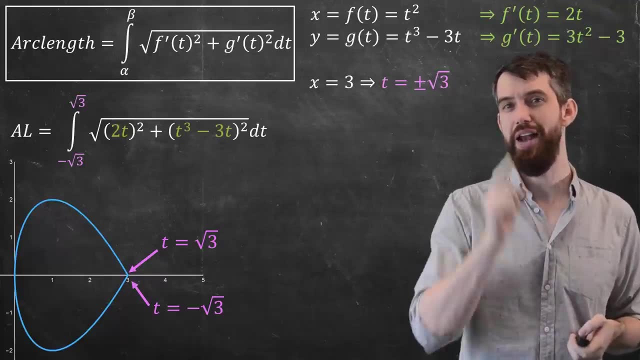 square root of the f prime squared and the g prime squared, and this is actually a super gnarly integral. I don't really want to do it, but I can do it numerically by going to WolframAlpha or whatever you prefer, and you plug that in and what you get is approximately 8.98, as